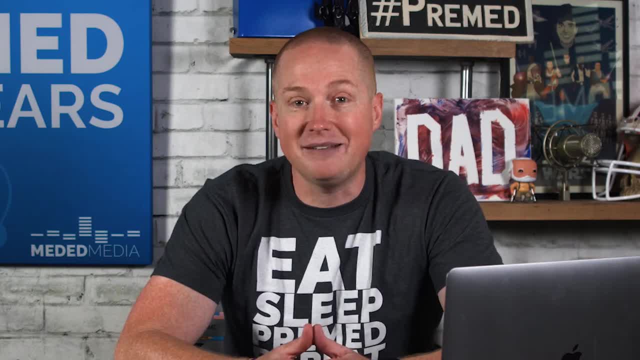 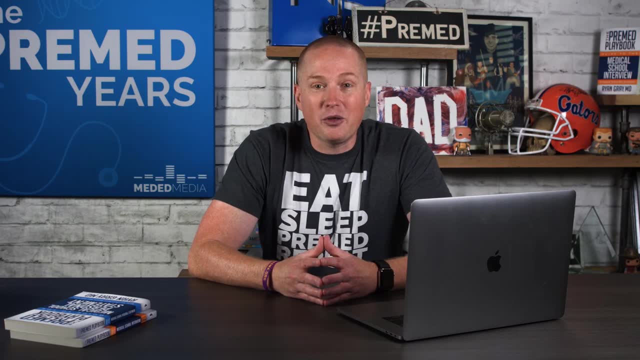 in my podcast, a site that has reached out to me for support for help to make them better. Unfortunately, that hasn't really gone the way I've wanted it to go, partly because I haven't heard much from them, So hopefully, after watching this video, they'll reach out to me and 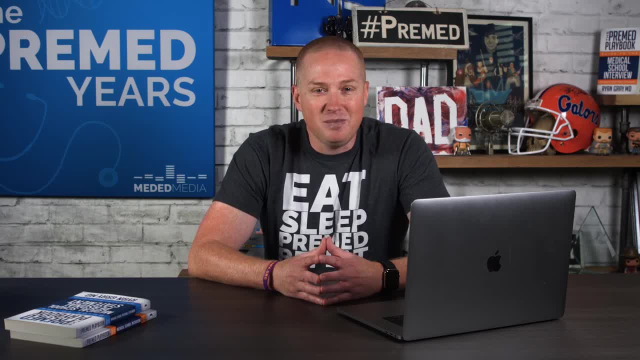 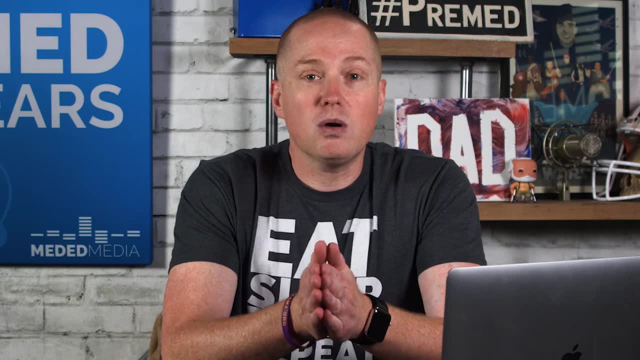 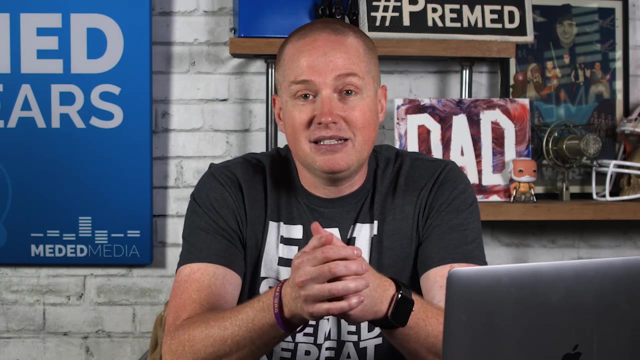 we can actually help improve them. I won't name them, but you'll know who I'm talking about, because today we're going to talk about the Lizzie M score. The Lizzie M score is a score that is found on student doctor network. It was created by a user on SDN called Lizzie M. 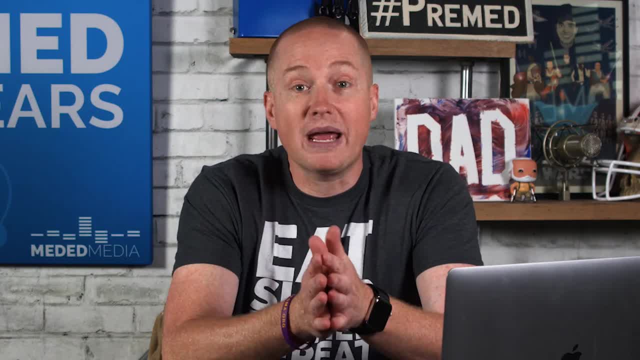 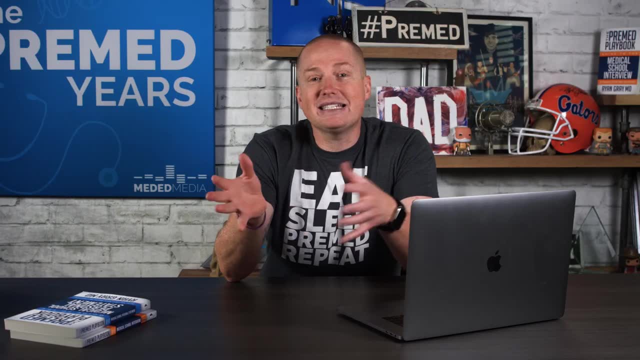 Now Lizzie M used to be the person who ran. Lizzie M used to be an admissions committee member at a medical school. I believe now that the sources that I have now say that Lizzie M is kind of a group of people now potentially at a different medical school or maybe different. 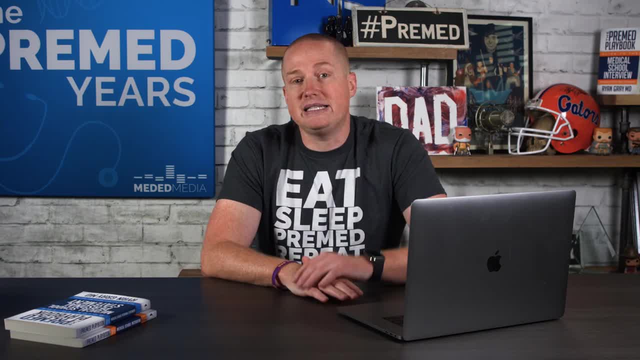 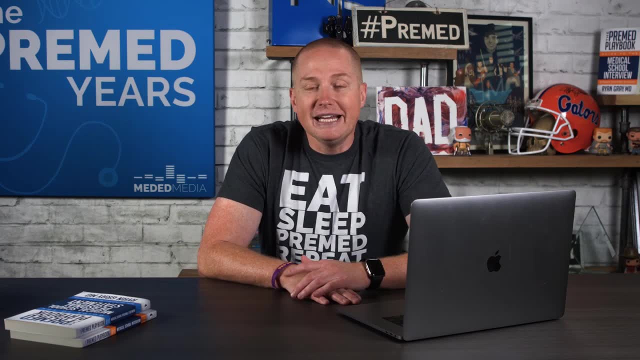 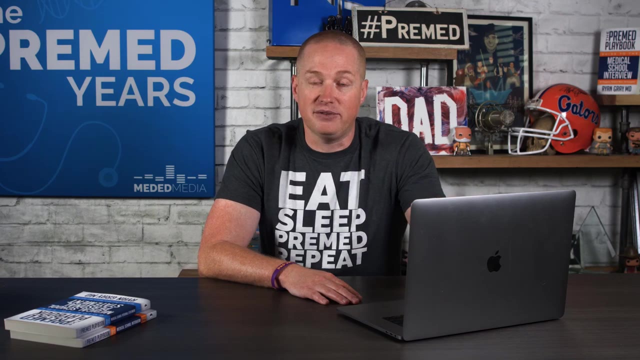 medical schools that run that account. And if you look at Lizzie M, you look at the advice that I'll say she, because Lizzie is a more of a female name, So I'll use she. If you look at her advice, really solid advice, advice that I would give the Lizzie M score. on the other hand, 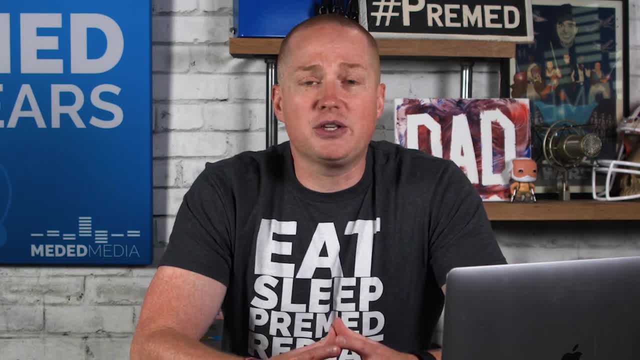 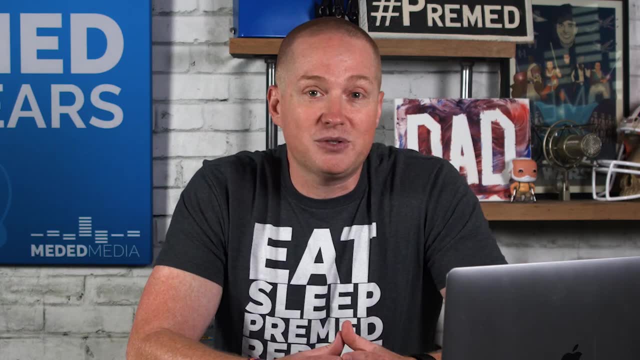 unfortunately, has grown to be kind of a beast of its own, And I actually covered this on the pre-med years podcast, episode 354, I believe, So go and listen to that. If you don't listen to my podcast, the pre-med years, I highly recommend you go subscribe there on Spotify. 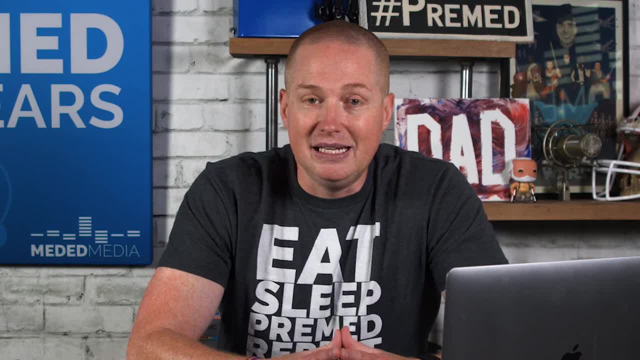 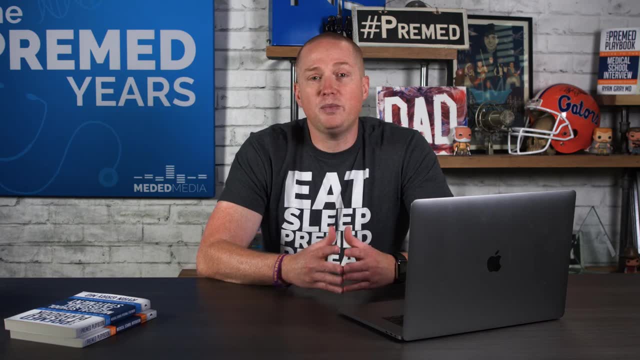 on Apple podcasts, on Google podcasts, wherever you listen to music or podcasts. So Lizzie M created this score And I think it's a really solid advice. And I think it's a really solid advice. I created this score some number of years ago as a way to potentially help students figure out. 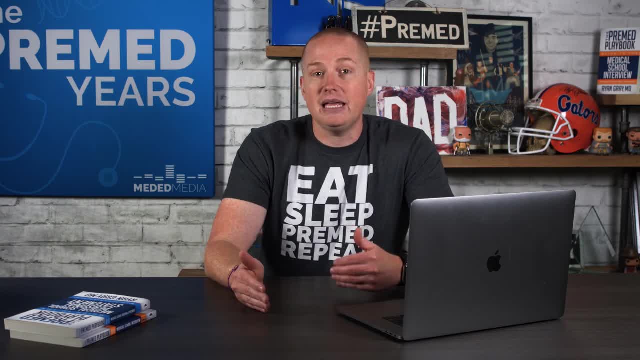 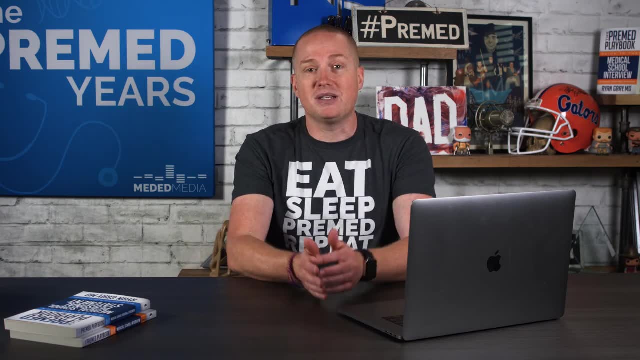 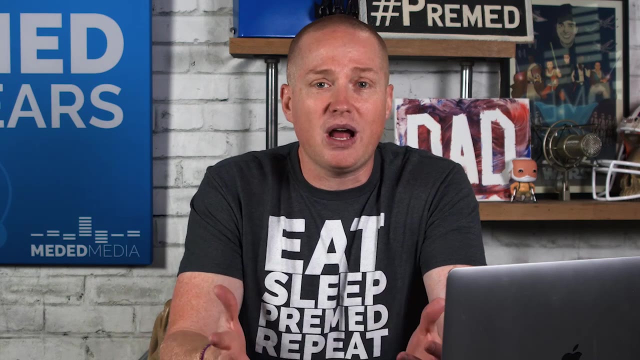 how strong their application is, how competitive it is right. One of the most popular things on Reddit on SDN, kind of anywhere among pre-med students, is: what are my chances? And the Lizzie M score potentially helps you figure out if you're competitive or not, but it really doesn't. 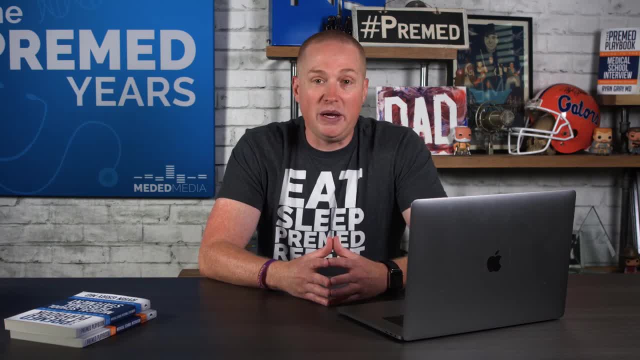 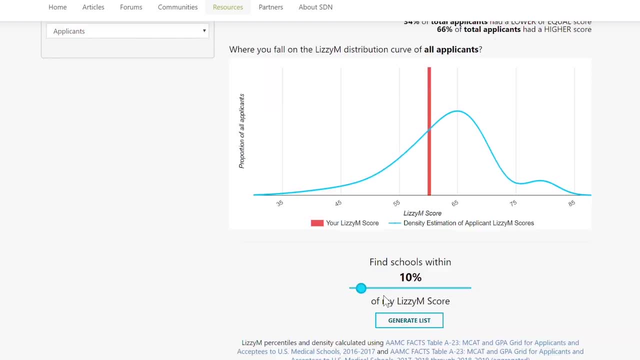 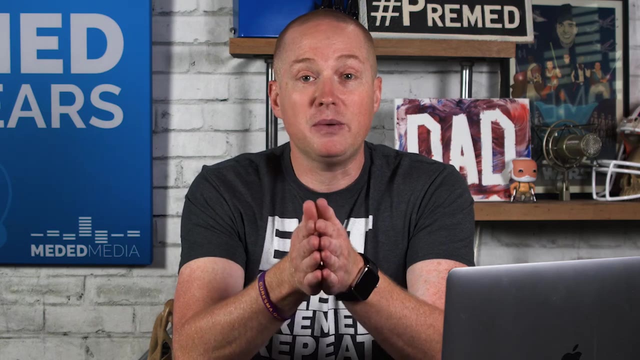 And let me explain why. Well, it's just a mathematical equation. It takes your MCAT score and takes your GPA and it mushes them together and gives you a score. And then, supposedly, what Lizzie M and what SDN and what other students would like to tell you is that then you can go. 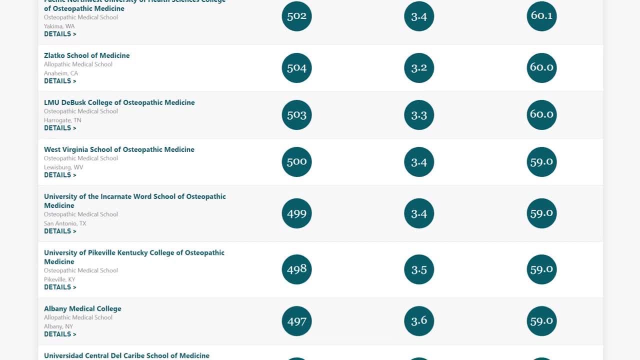 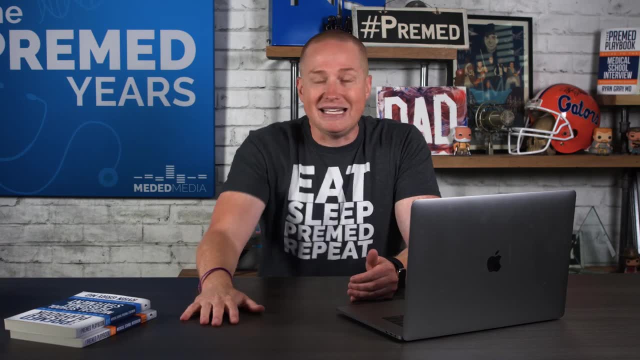 and you look at the schools and you look at what their Lizzie M scores are and you go: okay, I want to apply to this school and that school and this school and that school. Unfortunately, that doesn't work And it's garbage, because applying to medical schools is much more than just GPA. 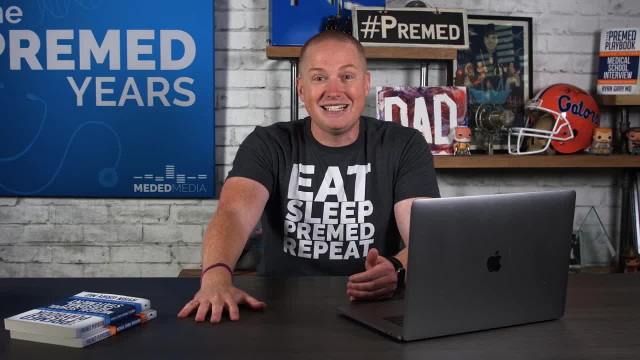 It's not just GPA, It's not just your GPA, It's your MCAT. It is, Trust me, it is Your story matters Where you grew up, the journey that you've been on, the hurdles that you've had to. 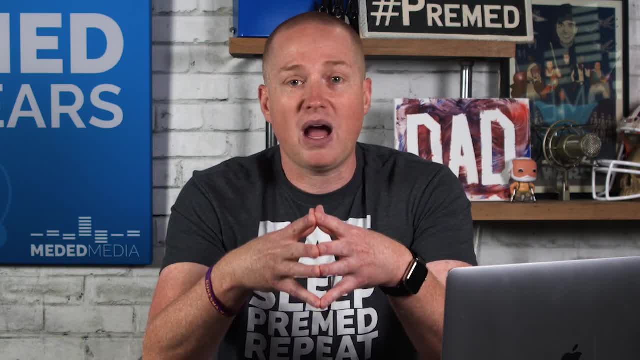 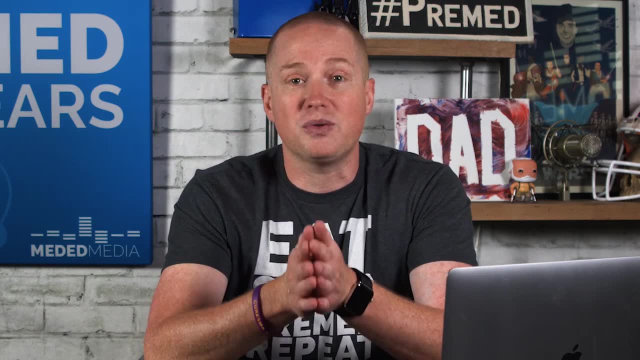 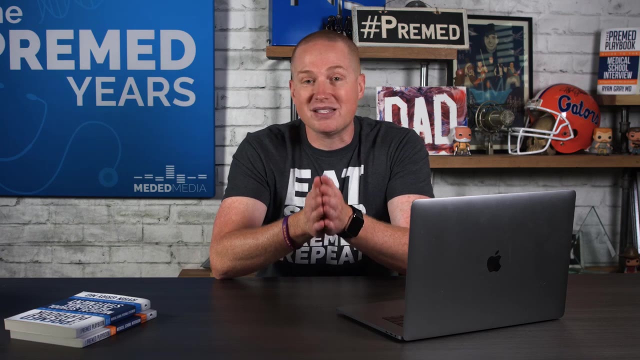 overcome your story matters. I've talked to enough admissions committee members, deans of admissions, directors of admissions to know that that's the truth. It's not just MCAT and GPA. Yes, your MCAT and GPA are important. I'm not saying they're not important, but they're. 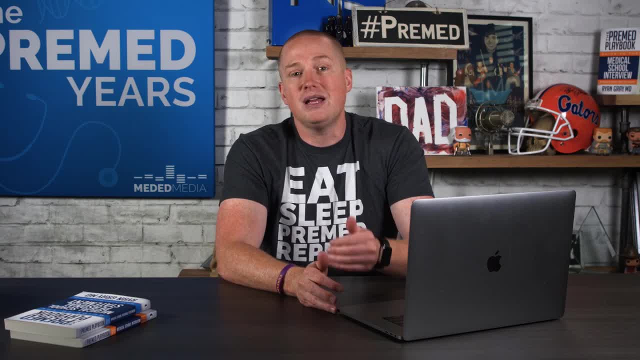 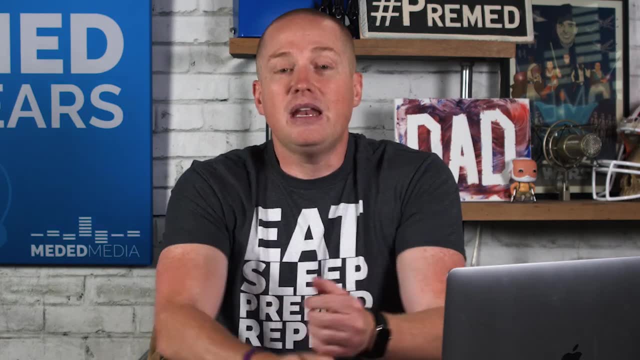 only important because they're important, because they're important, because they're important- And only important to a certain level- to get you into the door, to get your application reviewed. Above and beyond that, your story matters. Now, what is not often talked about with the Lizzie M score is 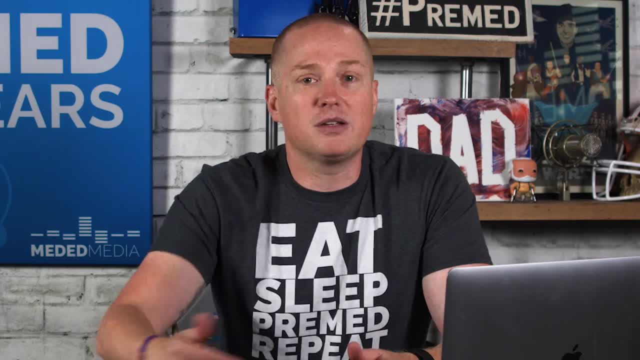 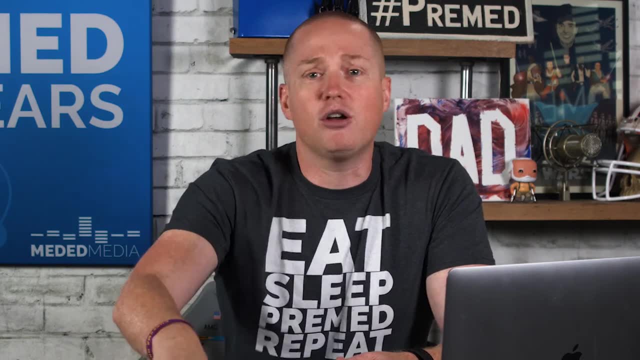 that medical schools aren't going to student doctor network. They're not going out to these other sites and going: hey guys, our Lizzie M score is X this year. right, Our Lizzie M score is going to be a cutoff of 70 this year. That doesn't happen. What the Lizzie M score is. 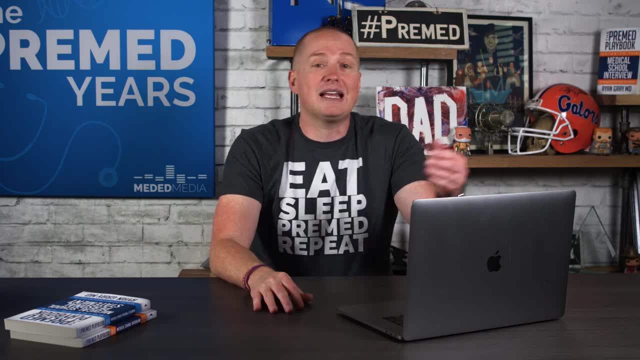 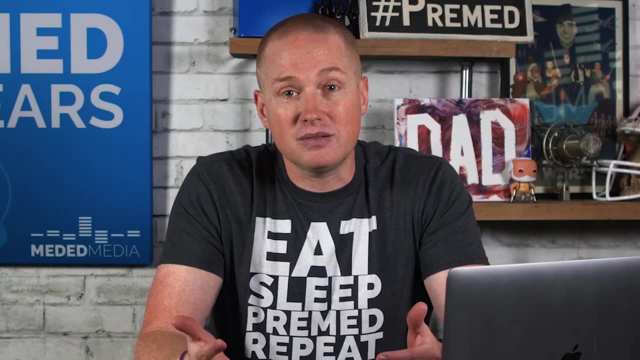 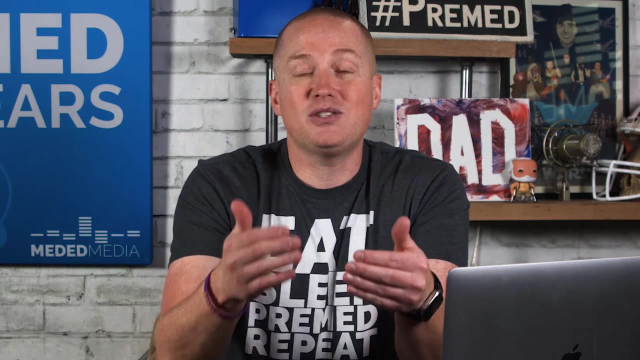 looking at is historical data from that medical school, looking at the acceptance class last year and the data that they have from last year. Unfortunately, that data is trash when it comes to figuring out where to apply to medical school, because all that tells you is what your GPA or 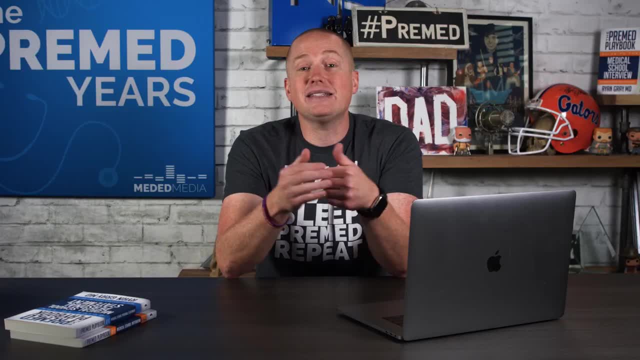 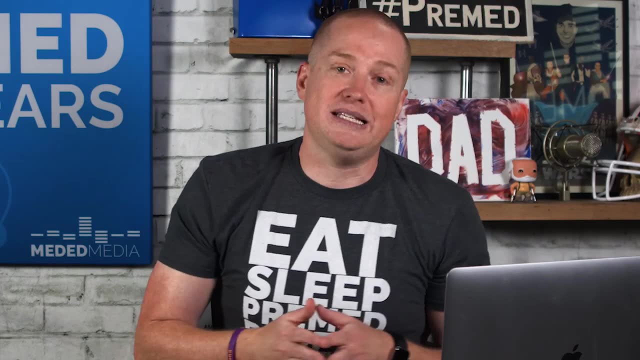 what their GPA and MCAT scores were for the class. It doesn't tell you anything about why those students were accepted. And so if you were trying to look at your Lizzie M score, taking your GPA, taking your MCAT score, and you're comparing it to the Lizzie M scores of 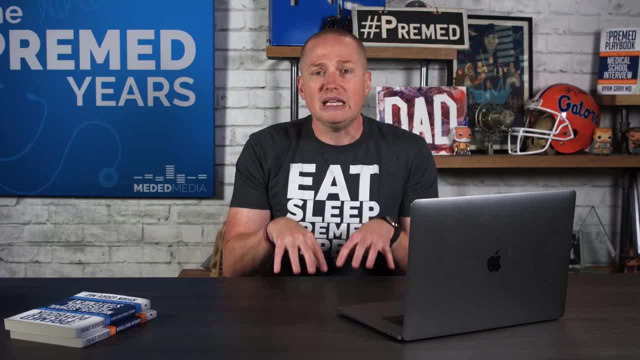 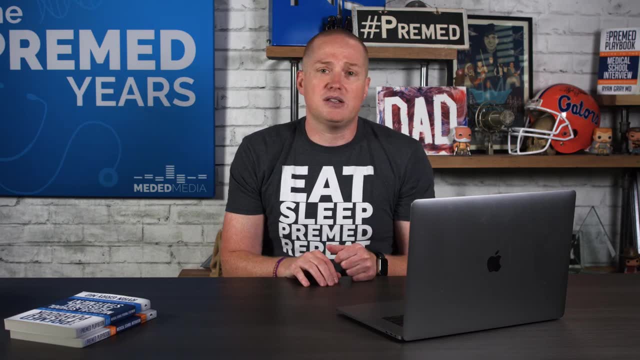 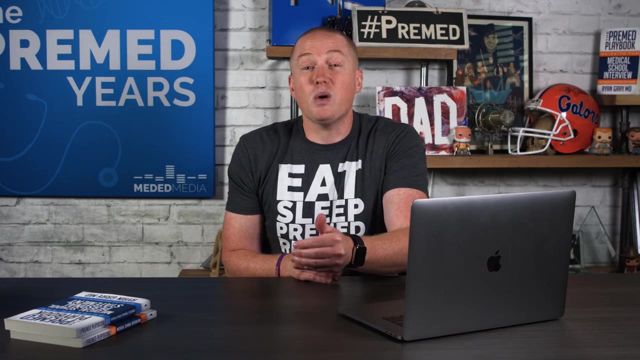 all of the other schools and figuring out where to apply. you're completely missing out on your story. You're completely missing out on your unique traits, your unique experiences. to compare those to the medical schools, to see if you are a fit for the medical schools. What do they want? 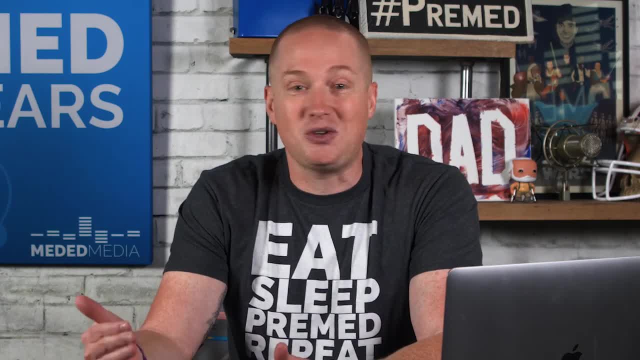 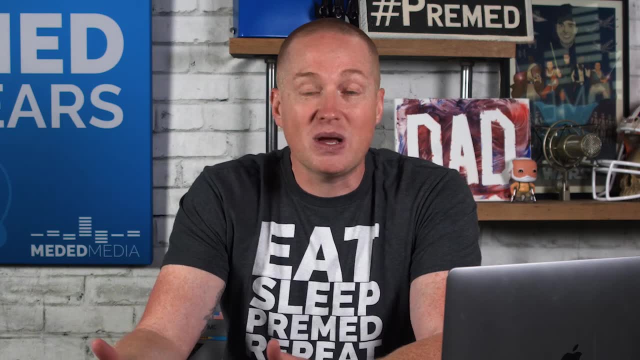 in a student. Obviously they want smart students, They want students. They want students that are going to pass medical school. hopefully in four years. pass the boards on the first try, go into residency, pass the residency exams on the first try and continue that cycle of producing. 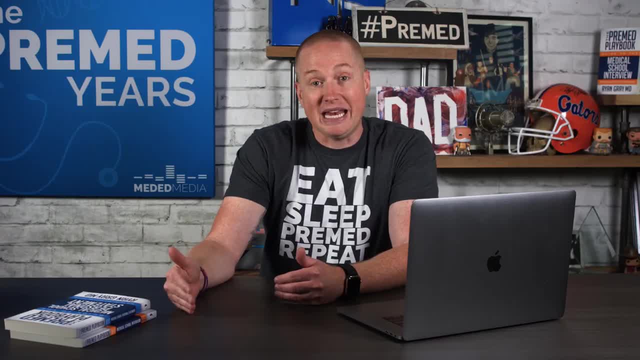 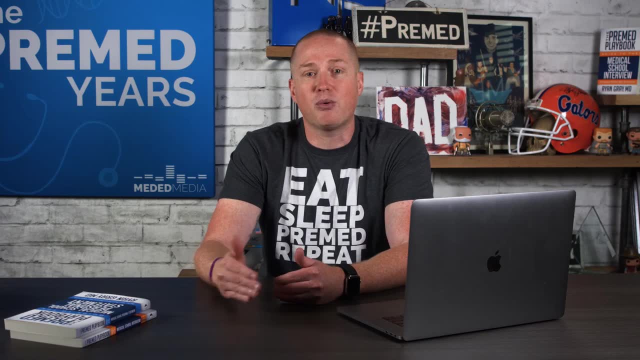 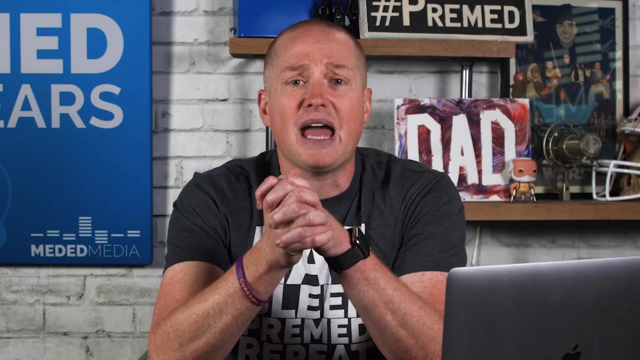 smart, competent physicians. That's why GPA and MCAT do matter. But above and beyond that, your story matters so much in the admissions committee process that you can't just look at one single score that mushes together your GPA and MCAT and go okay. 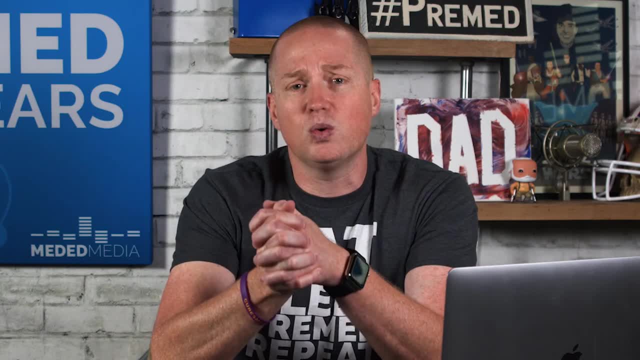 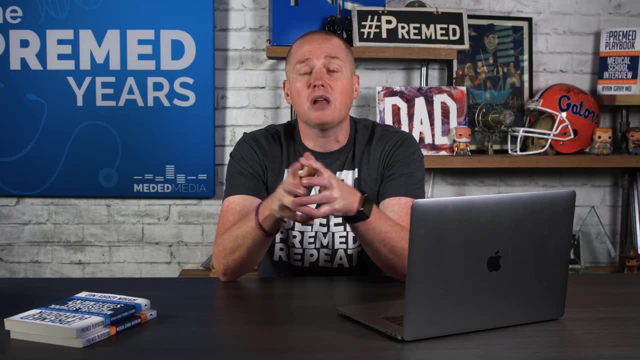 this is how competitive I am. These are the schools that I want to apply to. So when you are looking at applying to medical schools, know that you need to do a lot of homework. You need to look at the schools, look at their missions, look at their vision statements. 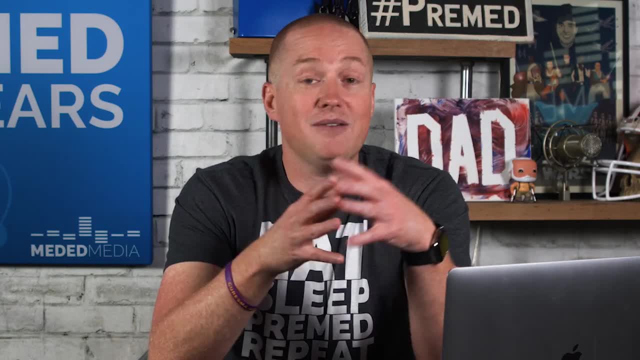 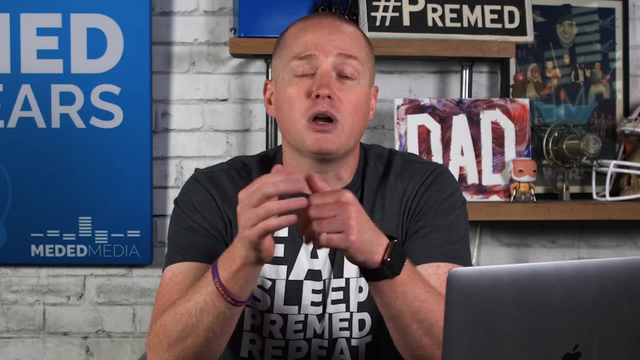 talk to students at the school. find out what their culture is like. If they have an open house, go there. talk to them. That's how you find out about the schools. Find out: if you are going to be a good fit, You need to have all of the good stuff that shows that you want to be a good fit. 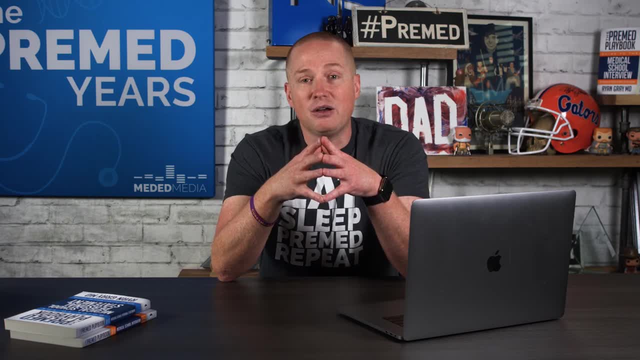 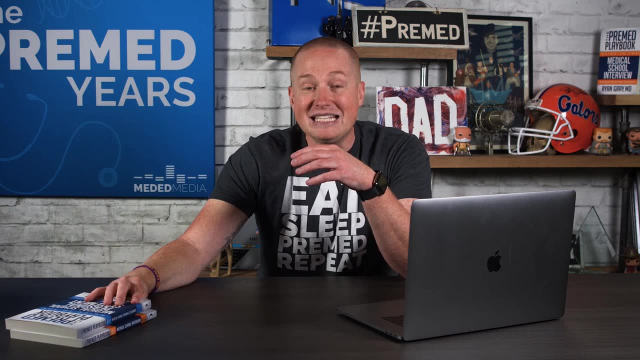 Like shadowing and clinical experience. You need to have a good story that you write about in your personal statement, which is why I have a book all about the personal statement, right, That is important and why I harp on it a bunch: Writing good essays for your secondaries, having a good 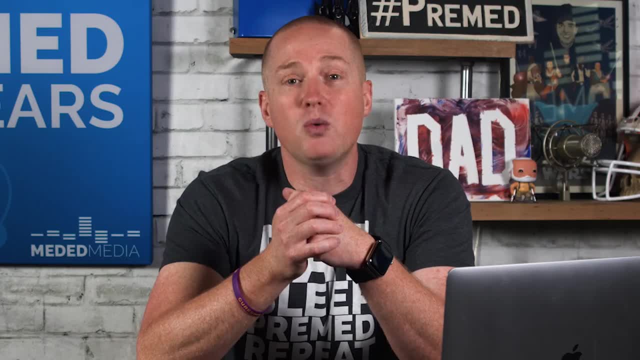 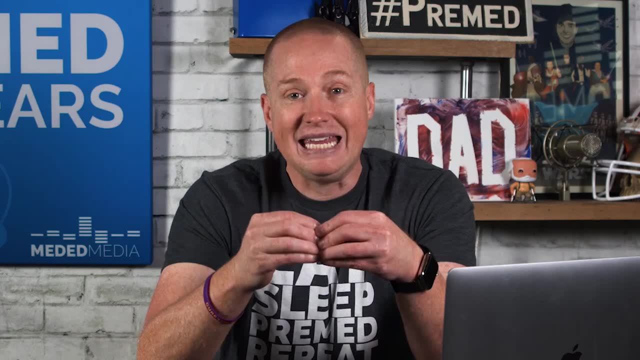 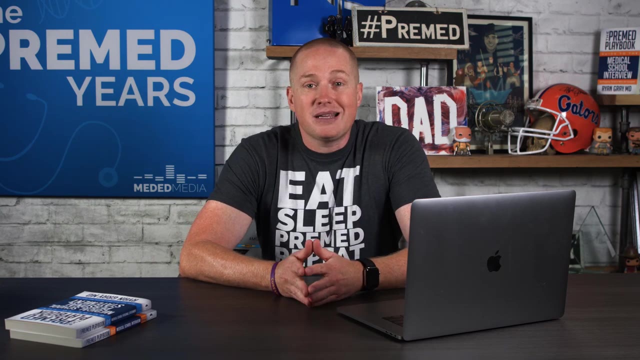 interview showing them that you are a good person. Don't narrow your application down into one single score. that doesn't mean anything. All right, guys, I hope that was helpful for you. Again, if you want more information, go check out the Pre-Med Years Podcast, episode 354. 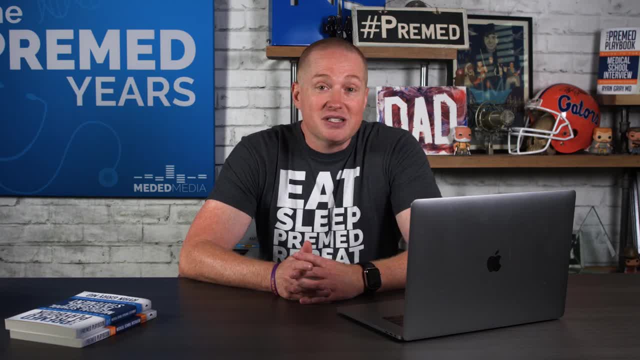 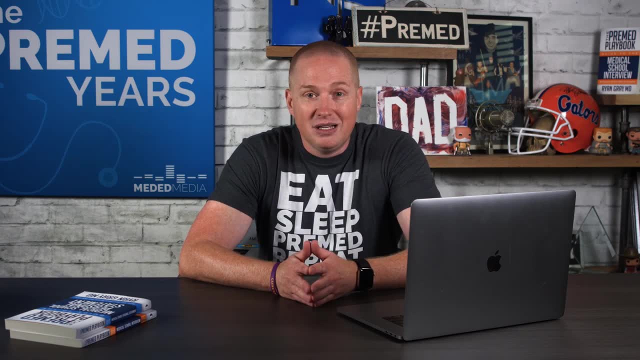 And for more of these videos, whether it's our Application Renovation Series, our Ask Dr Gray Series or whatever else we have coming down the pipe. don't forget to subscribe to this channel and let your friends know about it too. Have a great day.